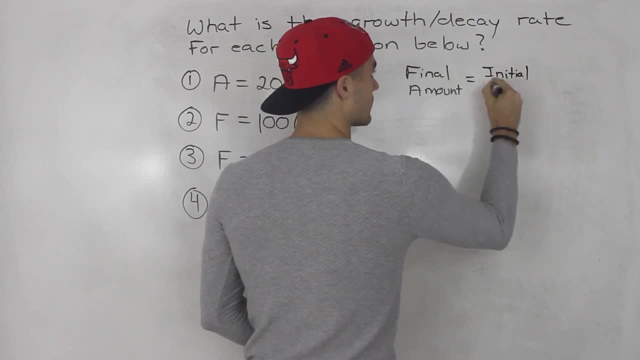 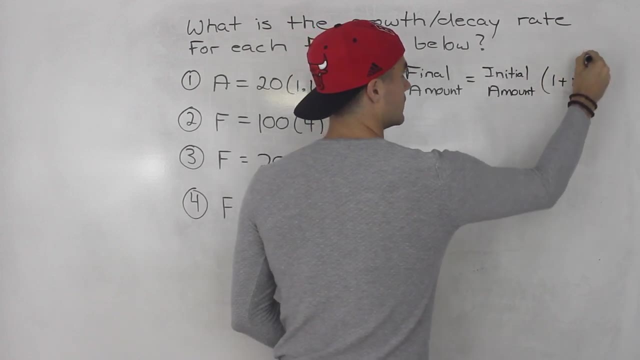 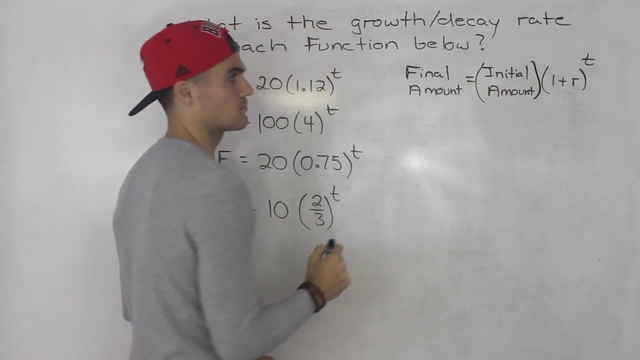 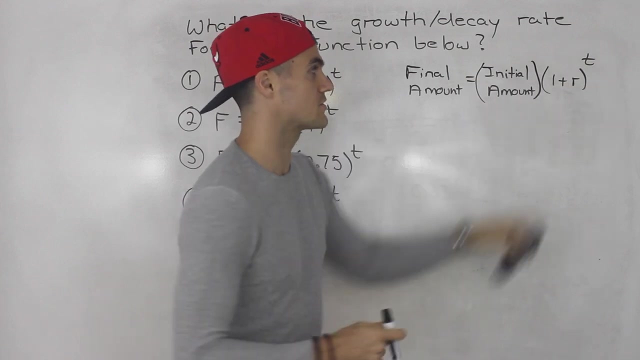 equal an initial amount or an initial value times 1 plus r to the power of a certain number of periods. So you're going to have an initial amount here, initial value in brackets, and then you're going to be growing it at a certain rate And it's going to be 1 plus r. So this here, this r, that is the growth. 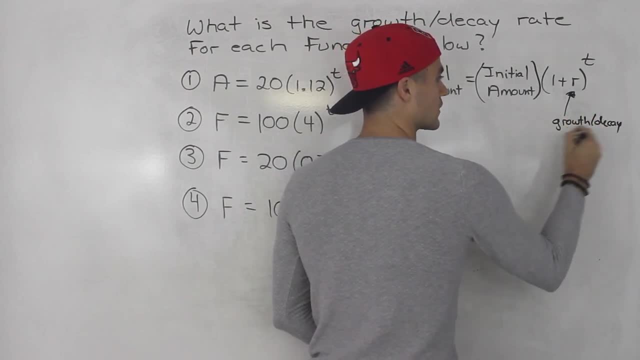 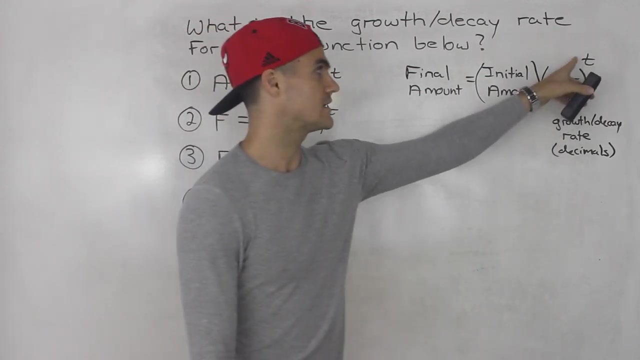 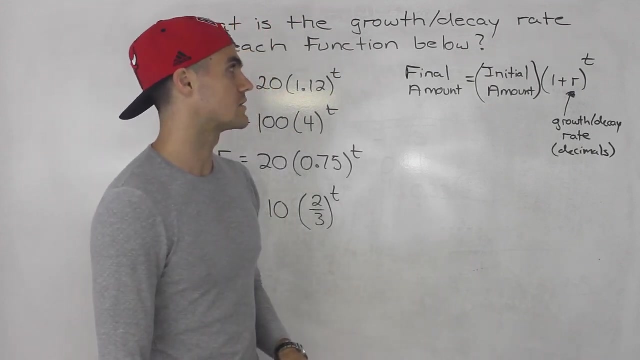 Or the decay rate that you're looking for. And remember, this here is going to be in decimals. That rate is going to be in decimals, So if you want to convert it to percentages, you're going to have to multiply it by 100.. And then t here is just going to be the number of periods, Either going to be growing per month, growing per year, whatever the question states. So this is the general format And notice. 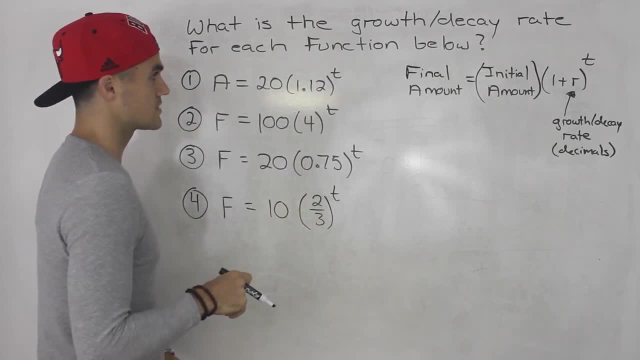 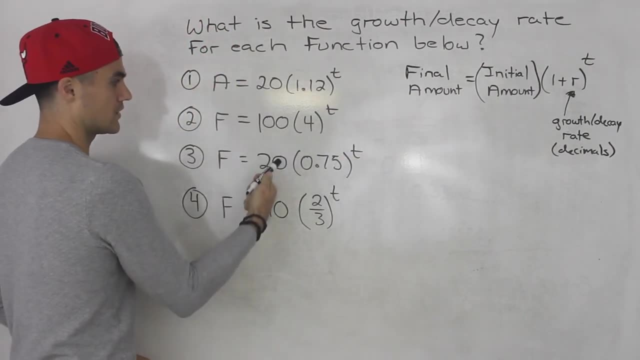 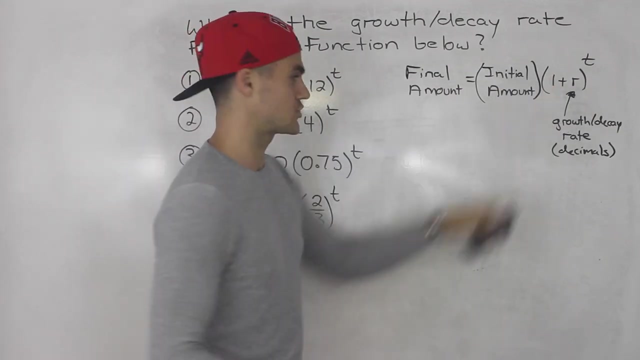 that all of these are in that format. So if this question was asking you what the initial amount is for each of these, well, easy to tell: It's 20,, 100, 20, and 10.. But they are asking for the growth or decay rate. So basically, we have to work with each of these brackets here. So pretty simple. All we do is we take this expression 1 plus r and we make it. 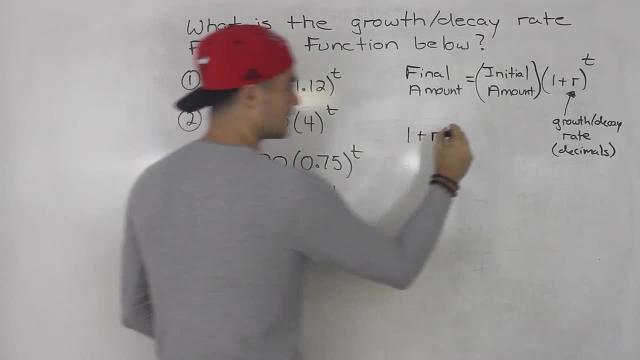 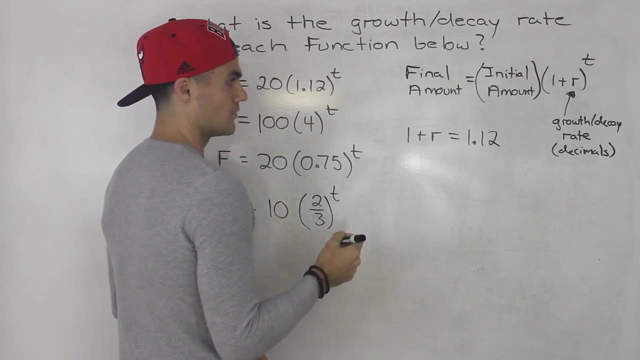 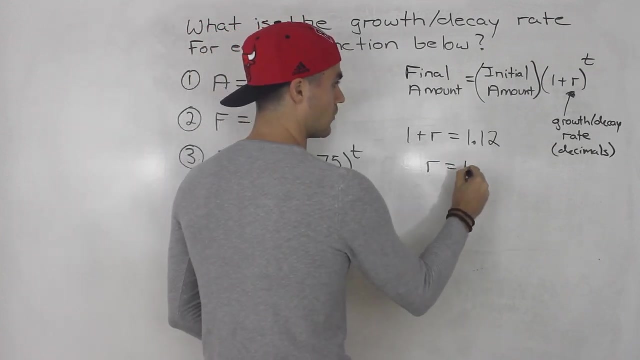 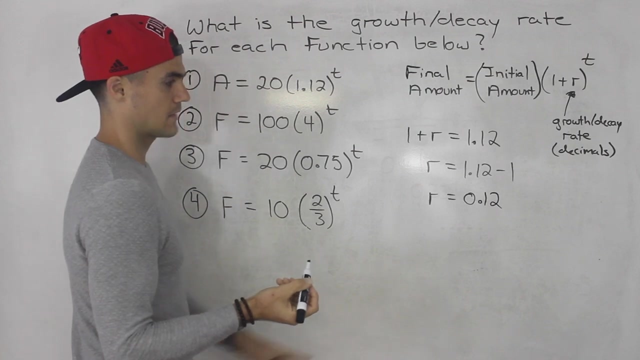 equal to each of these brackets. So, starting with this one, we make it equal to 1.12.. Okay, so here, bring the 1 over. r is going to be 1.12 minus 1.. So r is going to be 0.12.. Okay, and that's in decimals. So if you want it in percentages, multiply that by 100. 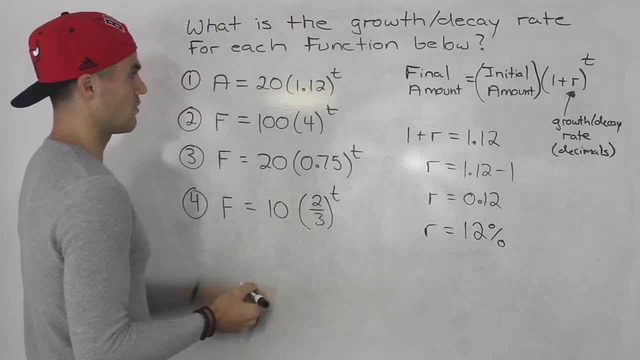 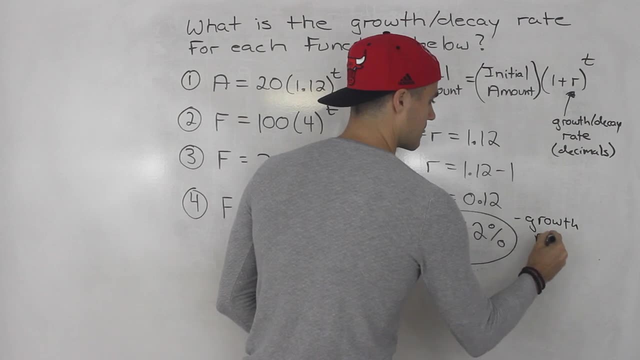 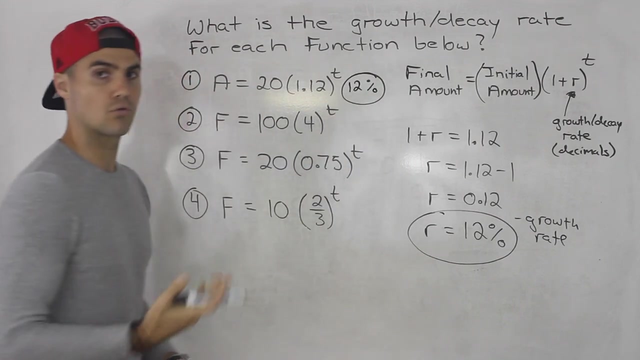 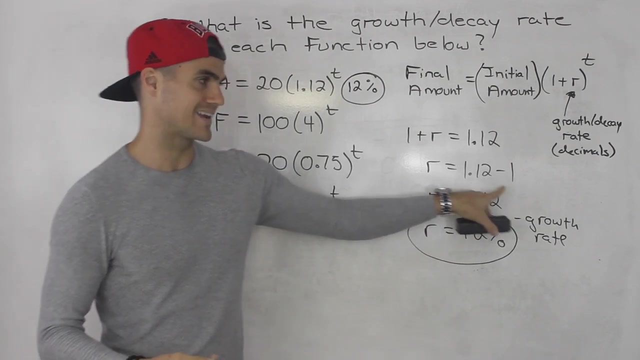 12%. So this function here has a growth rate of 12%. Now, how do we know that it is a growth rate and not a decay rate? It's because it's positive. Whenever you solve for this r value and it ends up being negative, it means that it's a decay rate. It means that 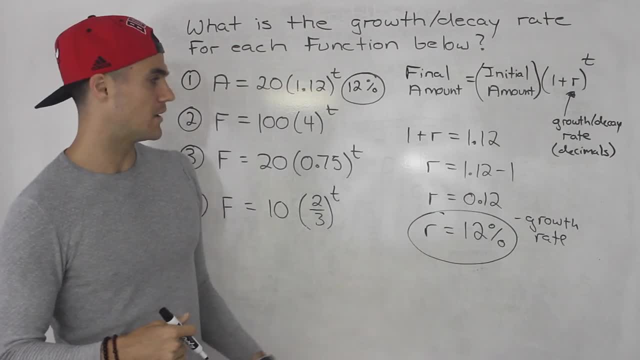 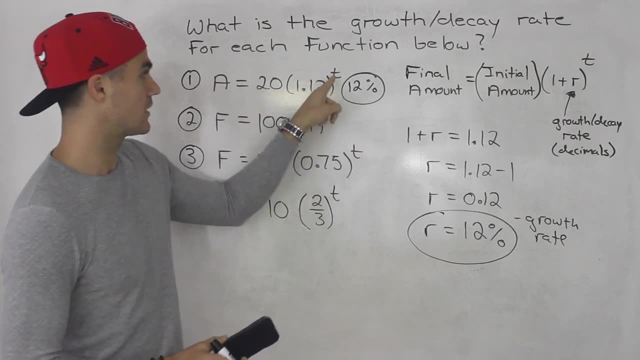 that initial amount of time is negative And then it sends us an error number. So if we, for example, amount is going to be getting smaller and smaller, but in this case, since we got a positive r, we know that in this case this 20 is just getting larger and larger if we keep plugging in values of one. 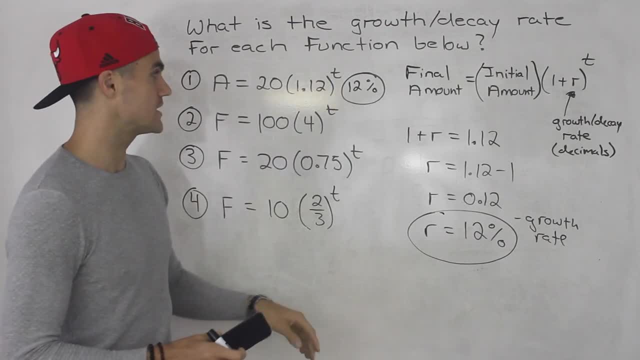 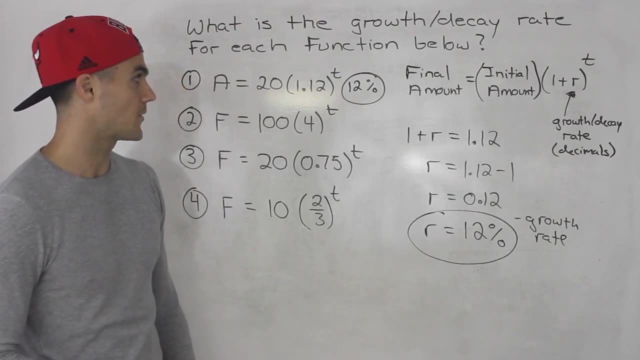 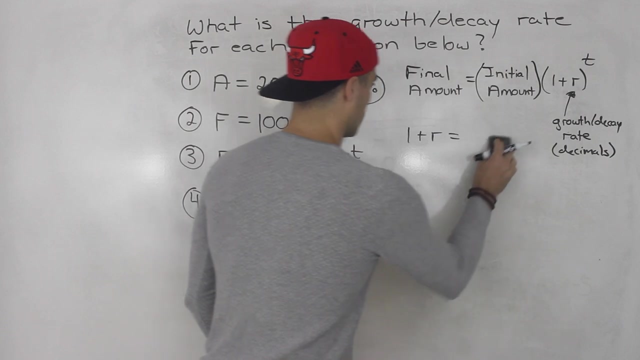 two, three, four, five, six, seven, etc. etc. for t, you're going to see each amount gets larger and larger. so that's when you know you're dealing with a growth scenario, right? so 12 is the answer for number one. now, what about number two? well, we would plug in four here, right, for that entire bracket. 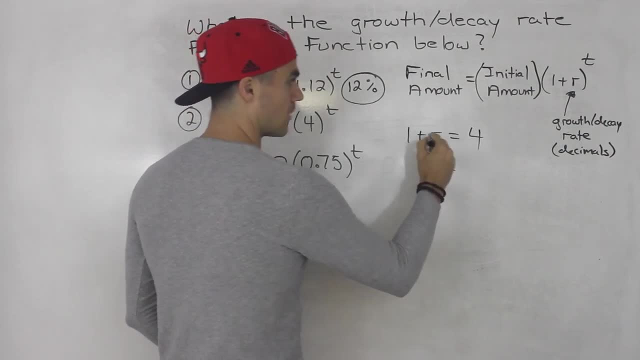 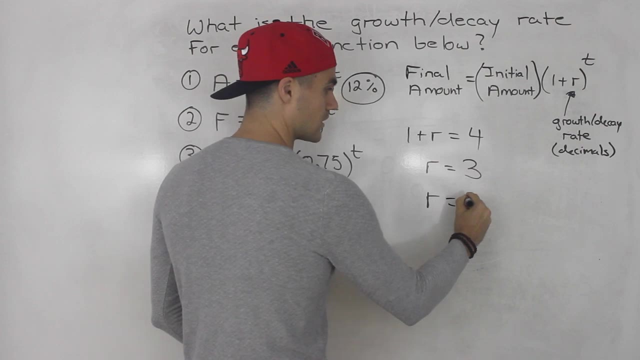 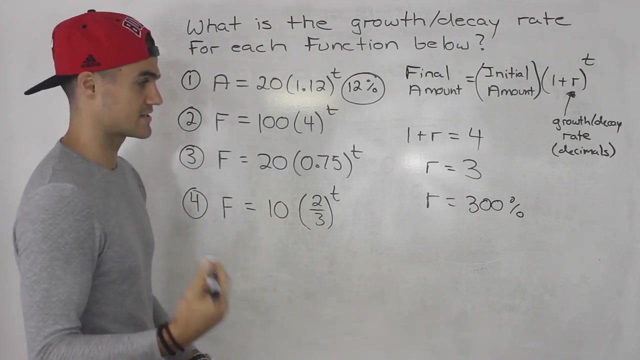 so here r would be what four minus one, which would give us three. remember this is in decimals. so if we multiply that by a hundred, it means that the growth rate is 300, and it's a growth rate because it's positive, you okay. so be careful with these whole numbers here. a lot of time you'll see two here, like something. 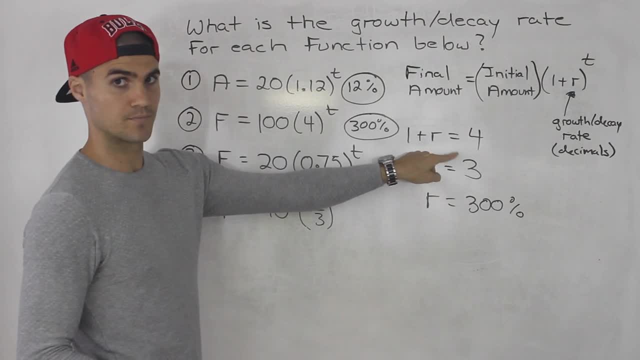 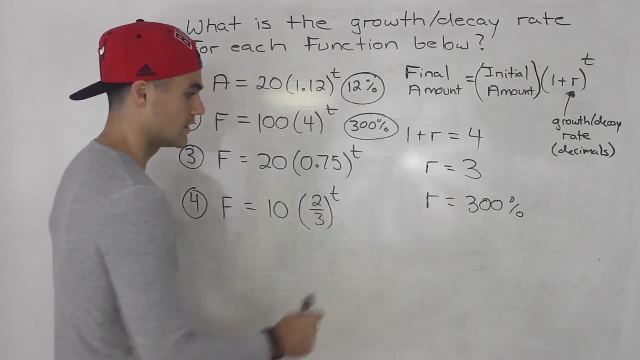 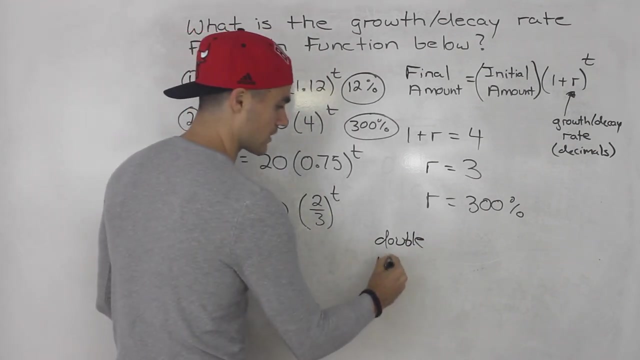 will be doubling. so if we had one plus r is equal to two, bring the one over, we would get r is equal to one. but we have to multiply that by a hundred to get it in percentages. so a hundred percent. so if something is doubling, it means it's growing by a hundred percent. right, that's the growth rate. 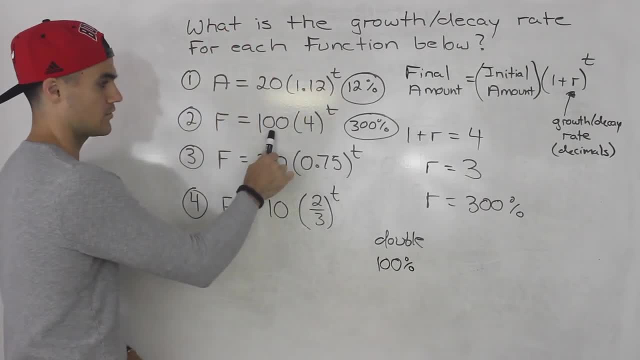 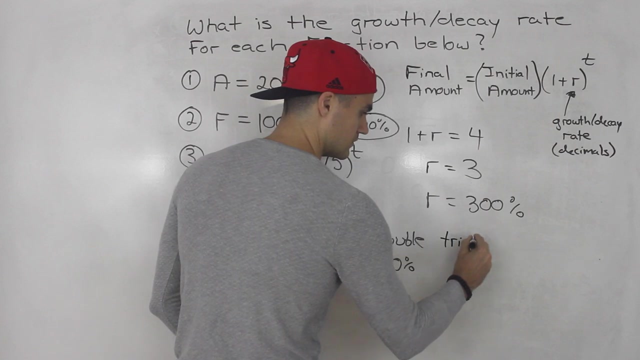 right? so let's say you start with a hundred and a hundred is doubling, then a hundred percent of a hundred is just a hundred. so you're adding another hundred on top of that, right? so if something is doubling, growth rate is a hundred percent. if something is tripling, right, growth rate would be 200 percent. if something is uh. 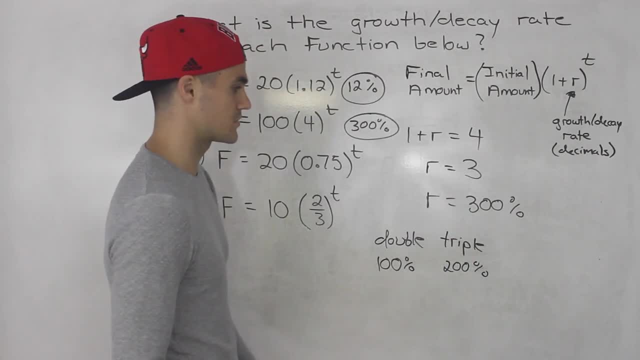 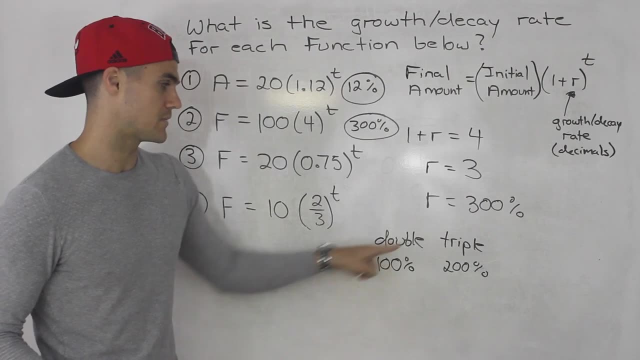 quadrupling, like in this case, growth rate would be 300 percent, right. so the growth rate is not 200 percent if it's doubling. that's a common mistake students make. they think that it's a doubling means that this has to have a two, but a hundred percent growth rate means that you're.